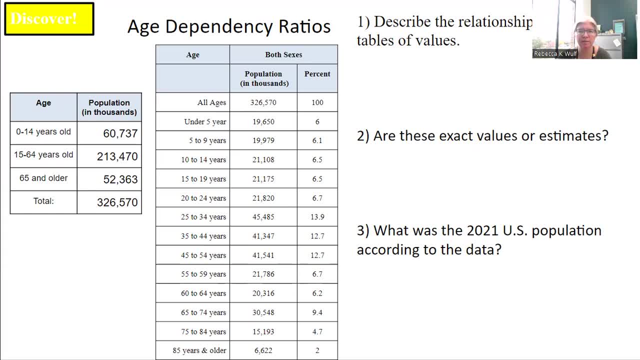 So this follows the book pages. in Section 2 on age dependency ratios, We see this table of census data from the government- actually two tables- And the first thing they ask us to do is to describe the relationship between the tables of values. And if you look closely you can see that the smaller table has combined some of those groups together. 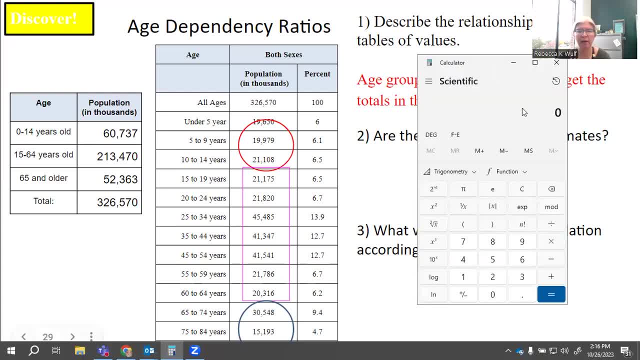 And they've just done that by adding up the values, So, for instance, 0 to 14-year-olds, they have added the under 5-year-olds to the 5 to 9-year-olds, to the 10 to 14-year-olds. 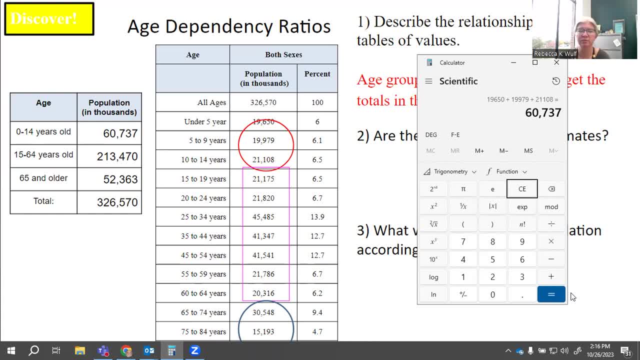 to get that 60,000.. So that's an 8,737 value. You could do that to put each of these groups together- And we're going to look more at these groups in just a second- but be thinking about why would you lump together 0 to 14.. 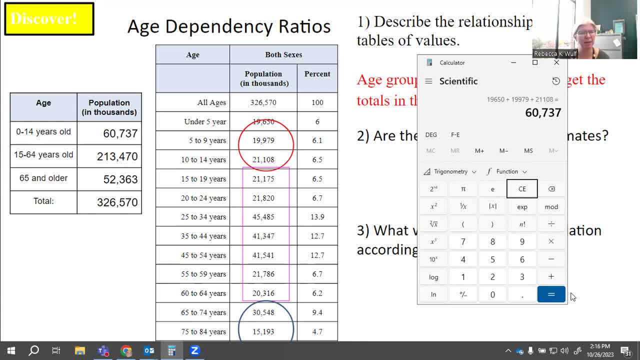 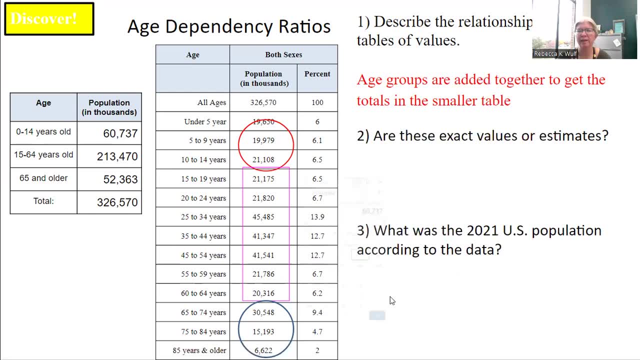 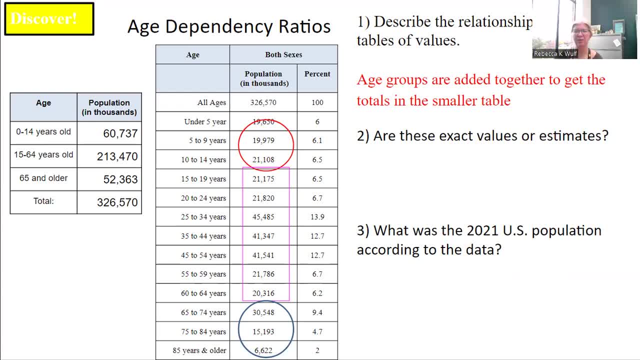 notoriously difficult to count. They move around. They don't want to answer their census pamphlets, things like that. So these are estimates And they want to know what was the US population? Well, I don't have to add all of these up. thank goodness They do give us the totals in. 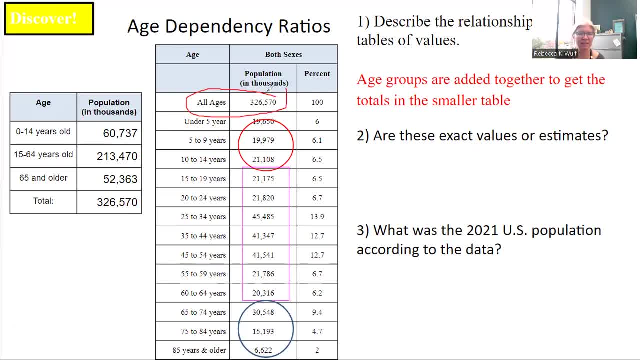 a couple of places. I can see here it says all ages And I can also see in the other breakout table where it says totals. So I see they match. Good, They should match. Those are the US population, Although, hmm, do those make sense for the US population, the entire population? 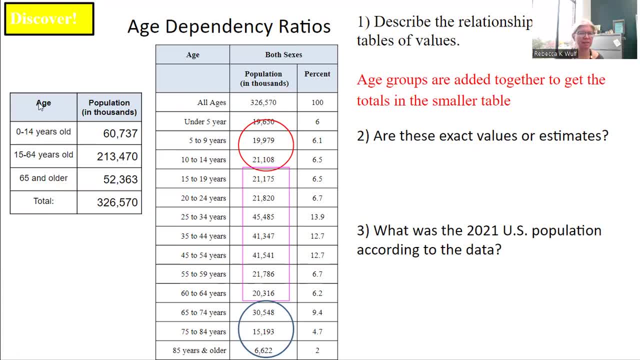 of the United States. Let's think about that. Let's use our quantitative reasoning: The entire United States has got to be way more than 326,570.. So what's the totals? What are we missing? So this class is a lot about attention to detail And there's a very small 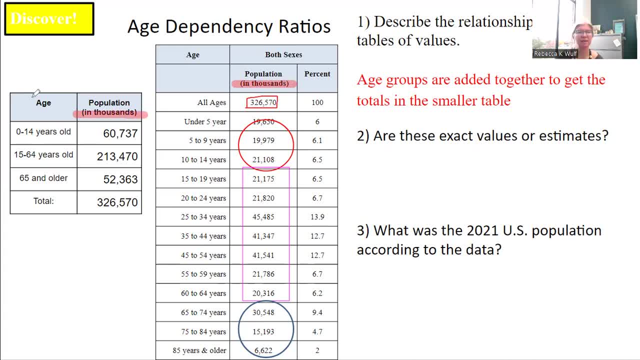 detail in both of these tables where it says in thousands. I know a lot of my students are like, yeah, 326,000, that's in thousands, Like no. what they mean is we have 326,570,000. 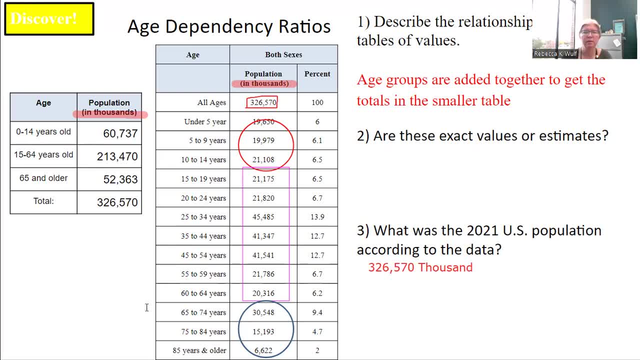 And let me ask you this: If I had 1,000, $1,000, bills, how much money would I have total? I wouldn't just have $1,000, right, I would have 1,000 times 1,000. I would have a million dollars. I wish I had a million dollars. 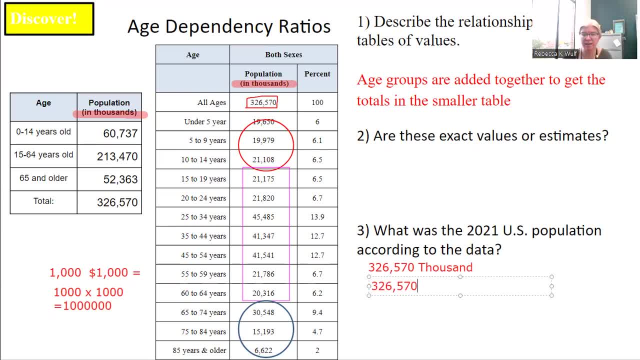 Here we have 326,570,000, means all of these values have an invisible 0, 0, 0 on them that they didn't want to put in the table. So I would have 1,000, I would have 1,000,, I would have 1,000,. 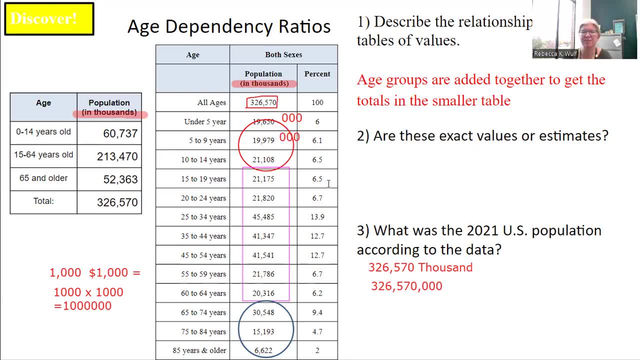 because they knew they weren't accurate to all those single digits. So they just kind of rounded them off and then didn't put the 0, 0, 0 and replaced it with the N thousands there at the top of the table. So what's a reasonable, meaningful answer for the US population? 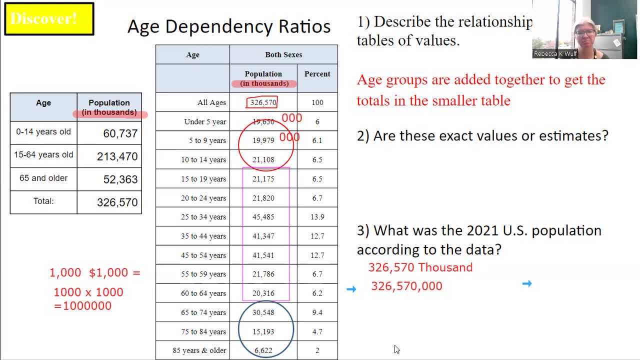 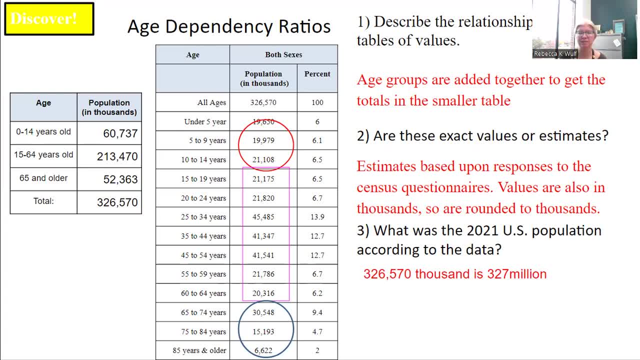 They're rounded to the thousands place, And then they just weren't showing those last three zeros. to save some space, The actual US population- we need to add those zeros back in. All, right now, let's get to the point here. The point of this section, section two, is ratios. So let's get back. 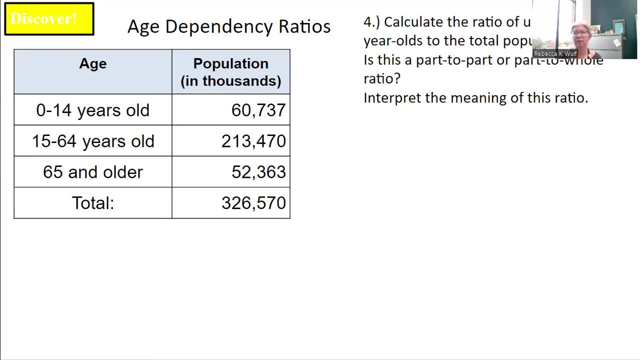 to calculating ratios. Number four asks us to calculate the ratio of under 15-year-olds to the total population, right Under 15-year-olds. that would just be another name for our zero to 14-year-olds, Wouldn't it? So let's take our zero to 14-year-olds. That's going to be the top part, the first part. 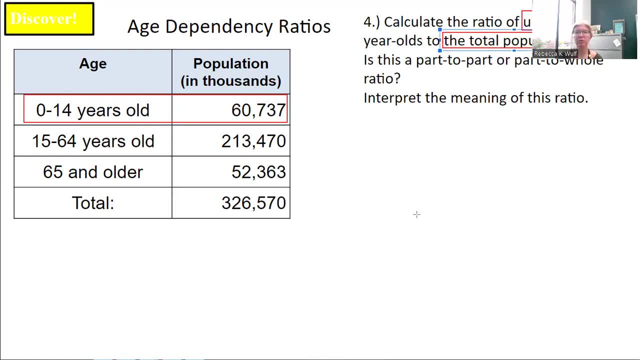 of our ratio. And then the second part of our ratio will be the total population which we just talked about. This would be a part to part or part to whole. This would be a part to whole. The zero to 14 are a subgroup. They're inside of the group. They're part of the whole group of the US. 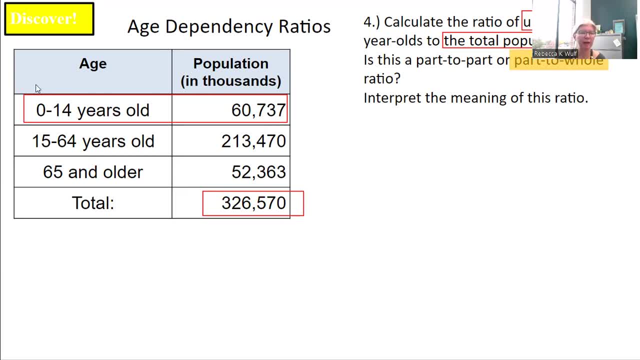 population They tell us to calculate. Maybe we should have been more specific here. So we want to take a ratio. We talked earlier in this section that there's lots and lots of ways to write these ratios, So we might start by writing them as a fraction. 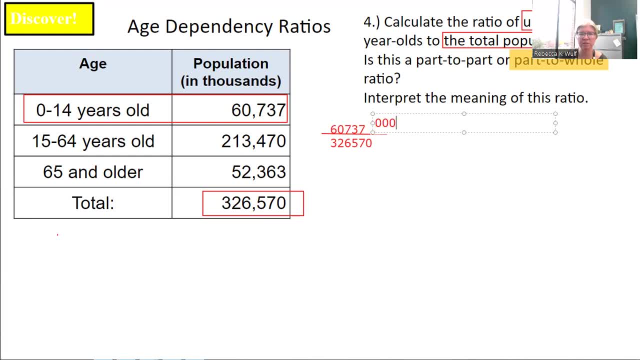 You may be thinking: oh, what happened to the zero, zero, zeros You were just going on and on about? They're still there. But I know that when I take this ratio they're going to cancel out anyway. So I'm going to take a ratio of one to one And I'm going to take a ratio of one to one. 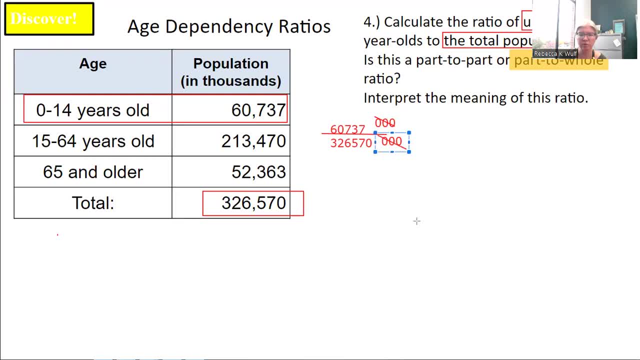 So you don't have to write them if you don't want to. They're going to cancel out And we're not going to leave our value as a fraction, And this fraction would also be way too hard to reduce. So we are going to divide and make it a decimal, And I don't see instructions. 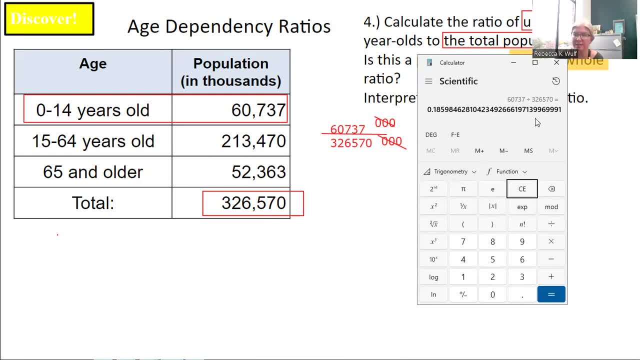 here, but we are going to round all of our decimals to three places, unless they tell us otherwise. So I have 0.18598, yada, yada, yada. The thousandths place is the five there. That's where I want to round to, So I look next to that. 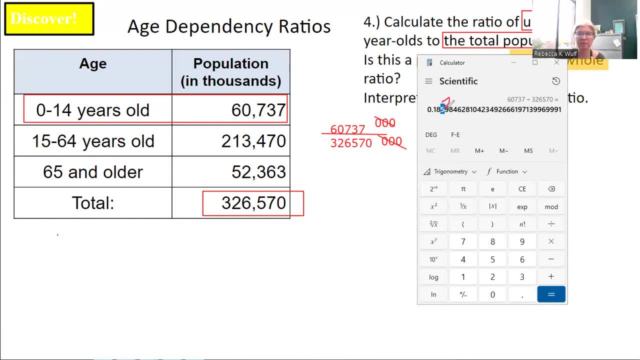 spot. I look just to the right, It's a nine, So I definitely need to round up And my final value will be 0.186.. That is my calculation of this ratio. Answer key guy agrees, And here's the important part. I'm going to take a ratio of one to one And I'm going to take a ratio of one to one. 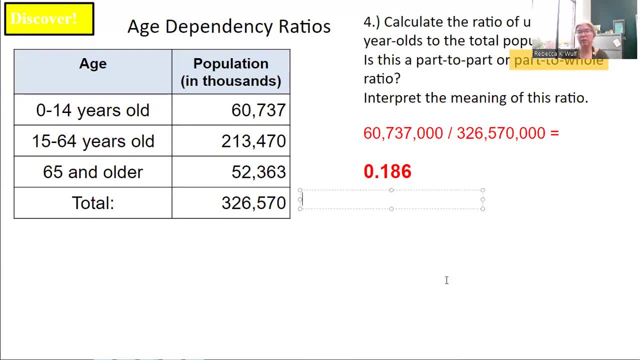 So what? What does that mean? Well, there's a lot of ways we can talk about this ratio, But when we talk about the ratio in a meaningful sentence, we're going to explain the meaning of this value in the context of the population here. So let's think about what our ratio was made up of. We 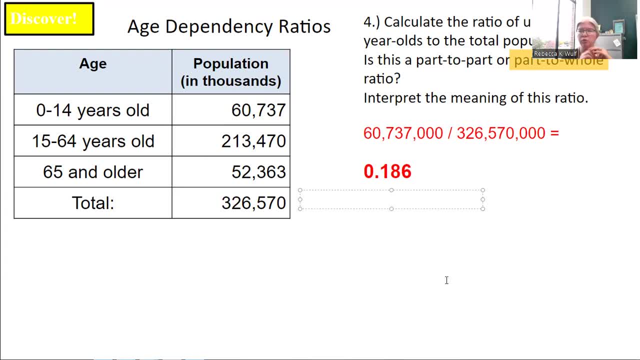 have our under 15 year olds and we have our total population. Those are two numbers. So once I make this a decimal, I need to have a second number here, And that second number is one. There's an invisible number, So I need to have a second number here, And that second number is one. And 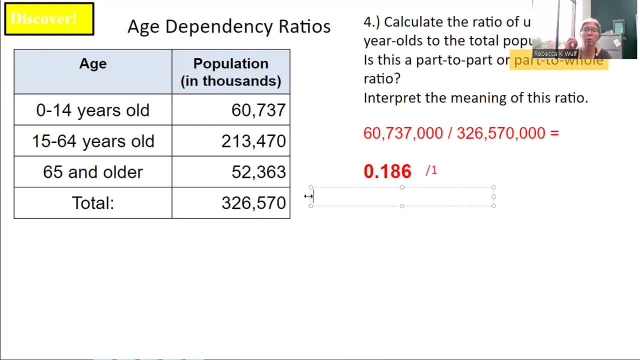 there's an invisible one here. So when we make something a decimal, it makes it per one. Now I could actually use 0.186 and one And I could say there are 0.186 under 14 year olds for every one person in the United States. I mean, I could say that That's perfectly fine. 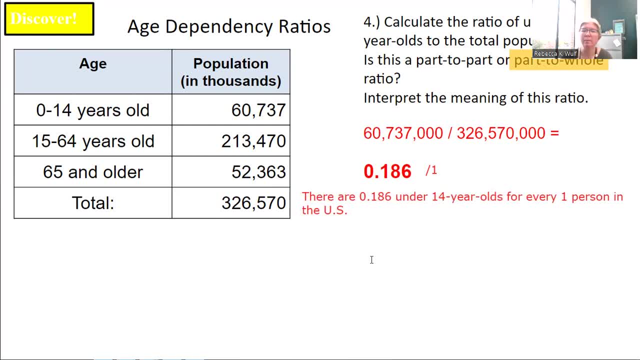 I think that's what Professor Becky did in her video, But I don't think that's very nice to think about 0.186 of a child. That's kind of weird. right? So we can scale these values by whatever we want, So I chose to round that decimal to the thousandths. 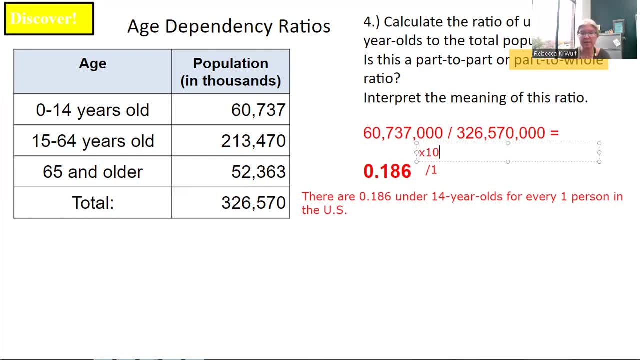 place. If I take this and multiply by a thousand, really multiplying top and bottom of this fraction by a thousand, an equivalent way of writing 186 thousandths is 0.186.. So I can say that's 186 over 1,000.. They're absolutely equivalent And that might make my statement a little bit. 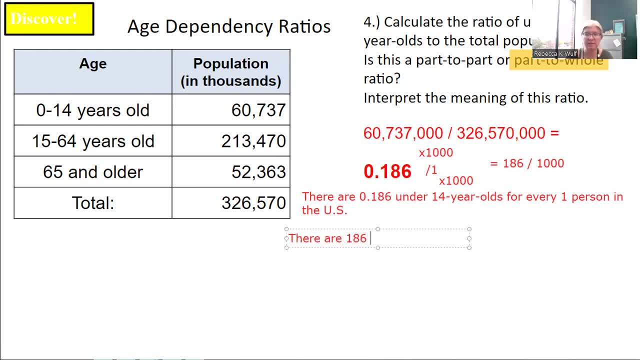 better. I could say there are 186 under. I'm sorry, under 15 year olds. I call them 14 year olds. I should say under 15 year olds. So 0 to 14, right, So they're under 15.. There's 186 under. 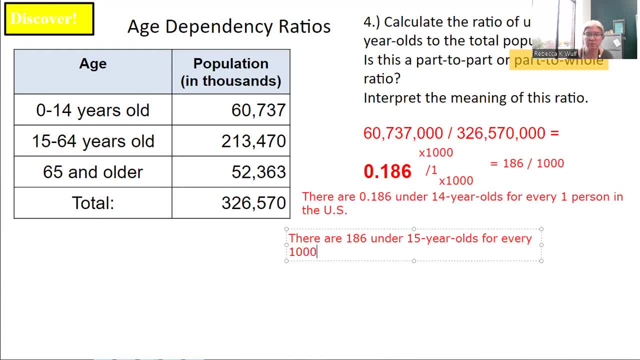 15 year olds for every 1,000 people in the US. Now this is a part to whole. Earlier the page on part to whole said we can make our part to whole percentages. So I also could make this a percent. Percent means per 100 to convert any decimal to a. 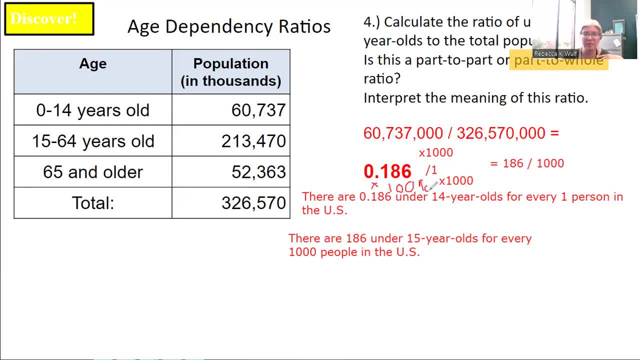 percent. We multiply by a hundred and we add our percent symbol. Multiplying by a hundred is the same as scooting our decimal two places to the right, So maybe even better sentence: Make it a percent: 18.6% of the US population. 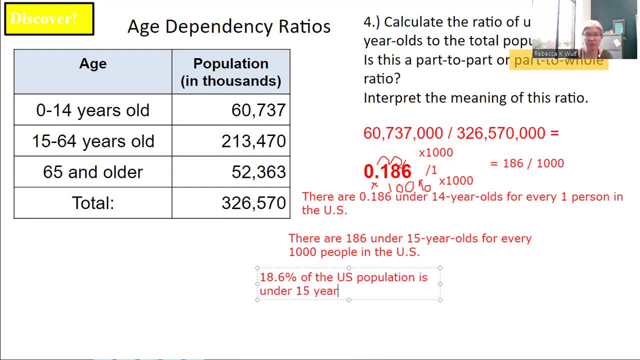 is under 15 years old. Now we can really picture that. Okay, about 18.6%, And we are going to call those child dependents here in just a second. Now that was a part to whole And we could scale it. 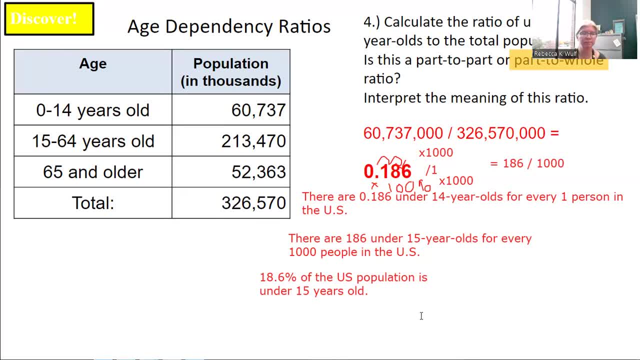 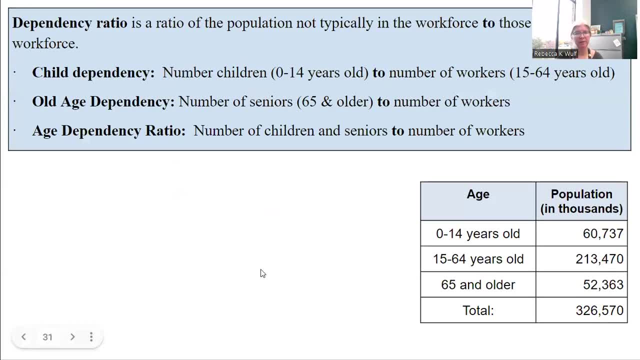 any way we want. All of these sentences are perfectly correct, perfectly fine. Actually, more interested in the next topic that we have here, Dependency ratios, And we have a box here, so it must be an important definition. Dependency ratio is when you take the ratio of a. 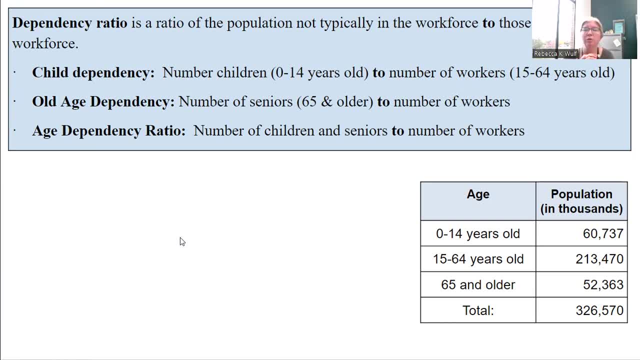 population who's not in the workforce to someone who is in the workforce. So if you are wondering why in the world did we lump together the 15 to 64 year olds, it's because we are going to consider those people working age. So those are going to be our working age And we're going to consider 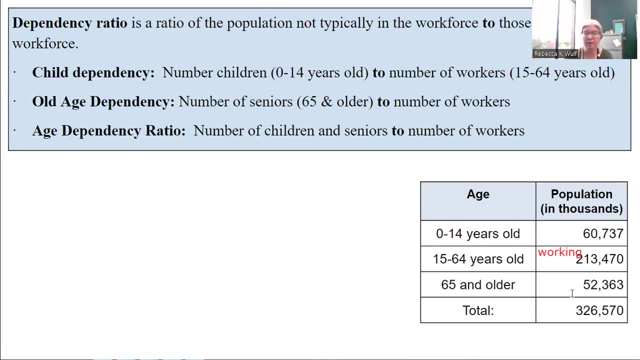 our working age people, The 0 to 14, we're going to call those child dependents. 65 and older. the government calls them old age. I always say that's rude. They're kind of our retired age persons. So the kids and the retired persons aren't working. The 15 to 64 year olds: 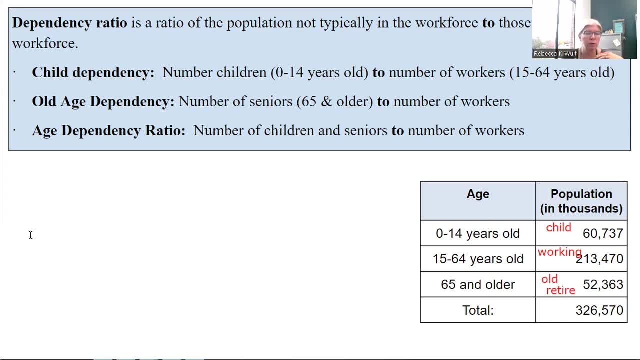 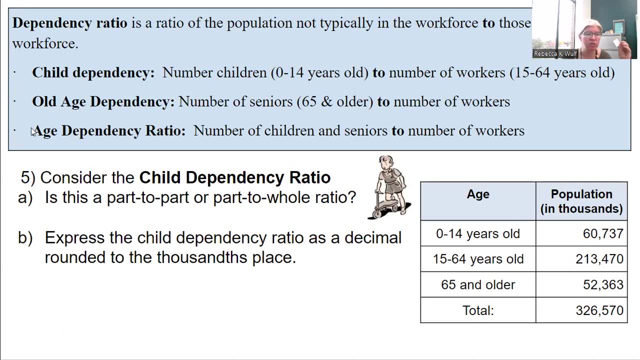 are working. We're going to have a couple different ratios we are going to look at. I'm just going to look at the first one: child dependency. So the child dependency ratio is going to be the number of people who are working in the workforce And the child dependency ratio would take the children. 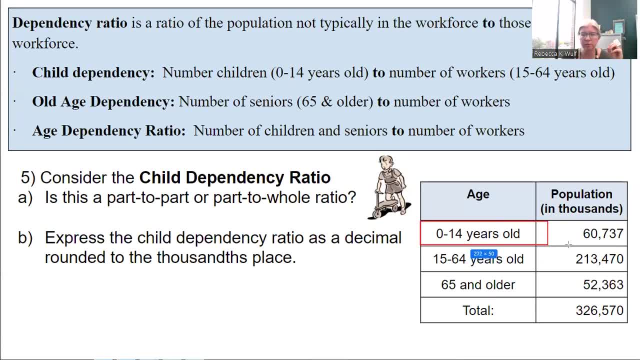 This is going to be different than the one we just did, because we're going to take the children and we're going to make a ratio, not with everyone, but a ratio with our 15 to 64 year olds. Why? Because we're taking the kids, who depend on the workers, and we're dividing by the workers, who 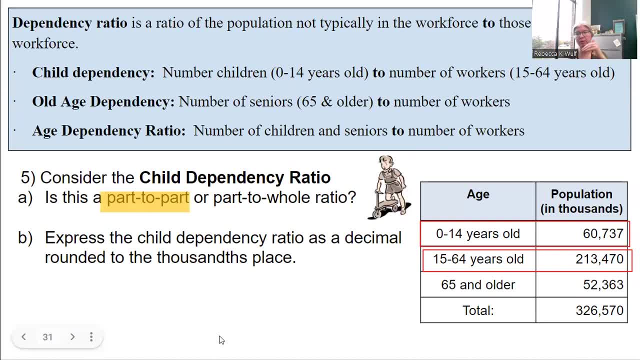 they depend on. This will be a part to part ratio. These are two separate groups that are not part of a part. They said we're going to take those children. divide by the workers, I get 0.285-ish again if I round to three places. Let's think about what that means. So what does that tell us? 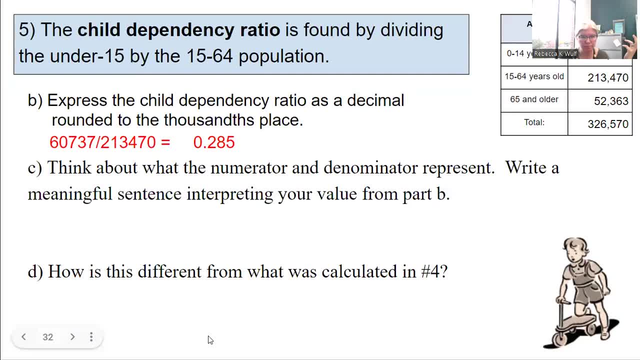 Well, think about what the values are. We took children and workers. Again, we could leave it in decimal form. We could say: we're going to take the kids who depend on the workers and we're going to give them a point. We could say: that's what balance this is going to be, So okay there. 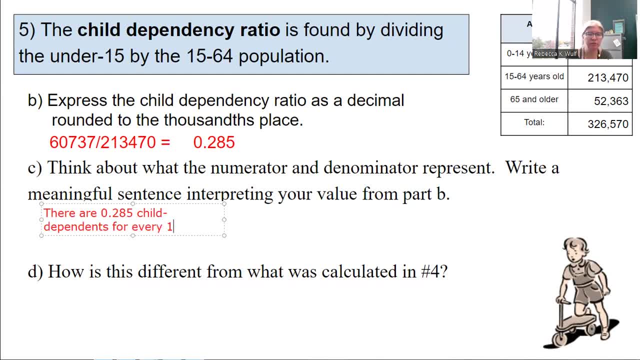 are 0.285 child dependents for every or for each one working-aged person. That sounds like a very technical sentence, but it's correct. So what's 0.285?? There's 0.285 kids for every worker, Okay. 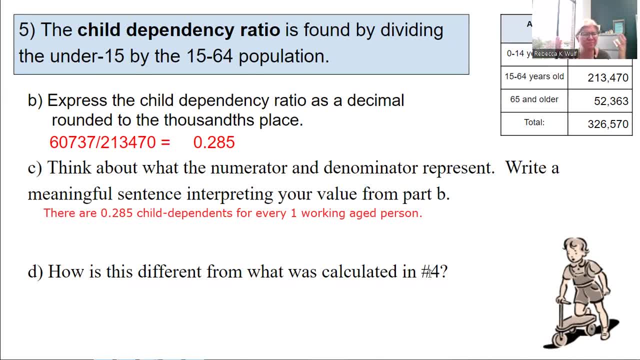 that's weird. That makes me picture chopping up people. I don't like that very much, But we could say that's what the value of the work per person is. Well, okay, that was great. Thank you both. Thank you. 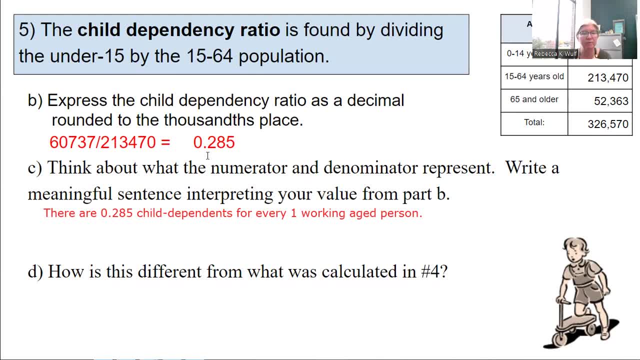 much I like to scale these values. I can scale by whatever I want: Ten, a hundred, a thousand, a million, Some power of ten is typically what we scale by. So 0.285, let's do, let's do a hundred again, Let's think about what that would mean. So if I 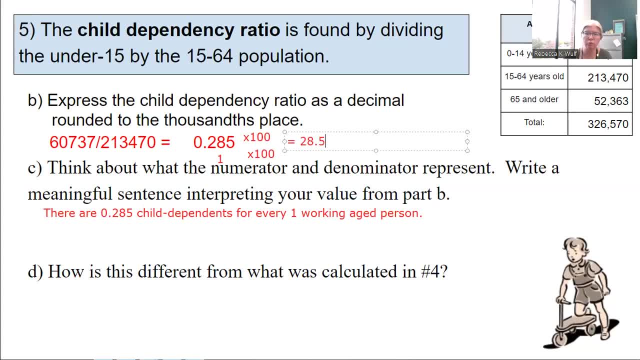 multiply that by a hundred, this decimal is equivalent to 28.5 out of a hundred. 0.285 is the same as 28.5 divided by a hundred. Or you want to stick with the thousand. you certainly can. That might make sense. If you want to round a little bit, you certainly can. So 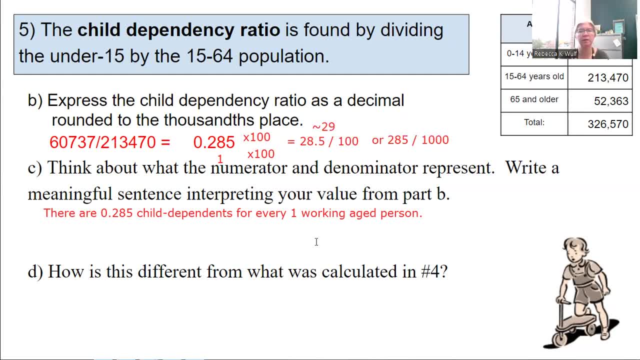 28.5, I can say that's about 29.. We'll be a little bit flexible here. We're going to write the sentence we want to write. I could say there are 29 child dependents for every 100.. I was going to call them workers. I'll be a little more specific here. They're working age. 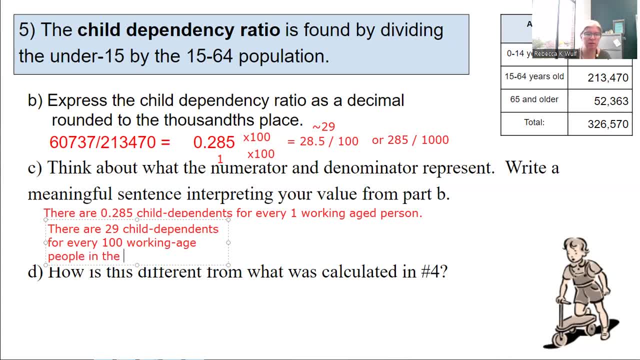 people Be even more specific in the US right, because it could be different in different places. Now notice what I did not do there. I didn't call it 29 percent. Why not? It's per 100.. Why didn't I? 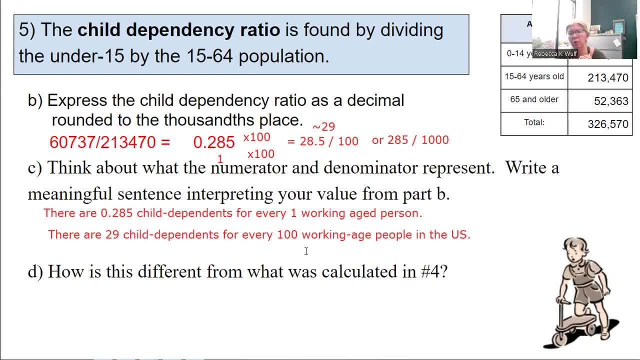 call it a percent, Because this is not a part to whole, So I want to be careful here. I could write a percent sentence and say something like the number of children is 29 percent of the number of workers. But I can't say something like 29 percent of the workers are children. That doesn't. 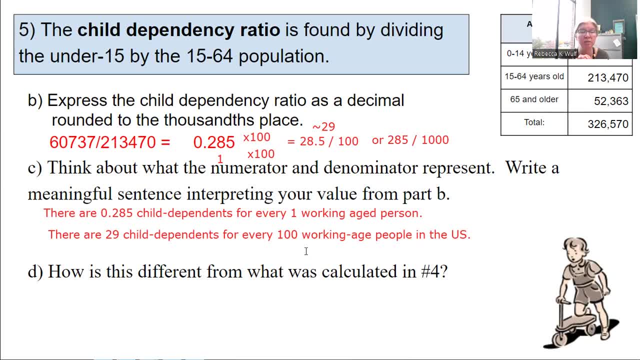 make any sense. I can't say something like that. I can't say something like that. I can't say something. 29 percent of the population is children. That's not correct either. We know from the previous problem that 18 percent are children out of everyone. This one's not out of everyone This. 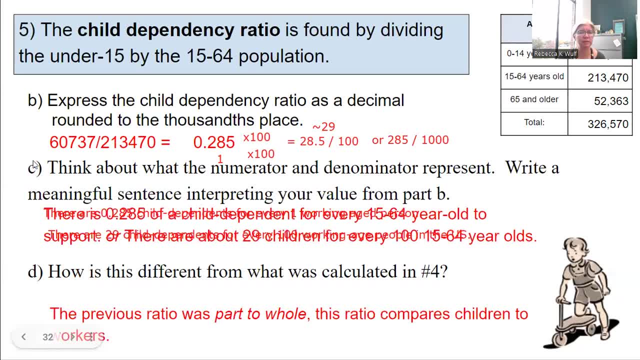 one is a part to part. So that's our big difference here compared to number four. Now we have a different denominator. Now we're looking at part to part. So per for each, for every, is a better way to state the value. Now for my students, as you look at the denominator, you're going to see that 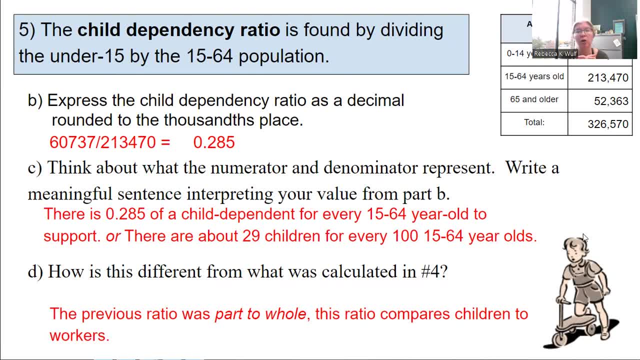 you have to pick from sentences And that is always hard because you're reading someone else's sentences. But I want you to look really, really, really closely at the descriptions that those numbers are attached to. Are they saying workers? Are they saying people? Are they saying children? 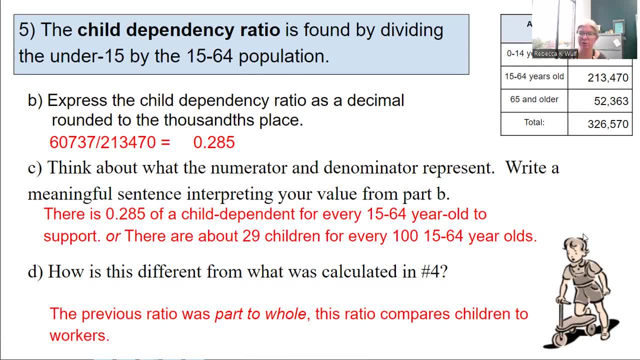 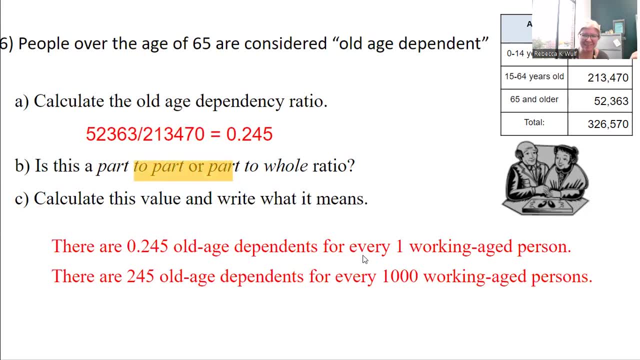 Is it the right group of people that they're attaching those numbers to Now? we could do the exact same process for our old age folks here. We could do the exact same process for our old age folks here. We could do the exact same process for our old age folks here. 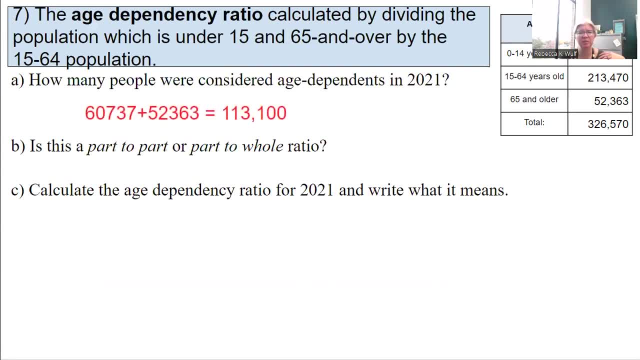 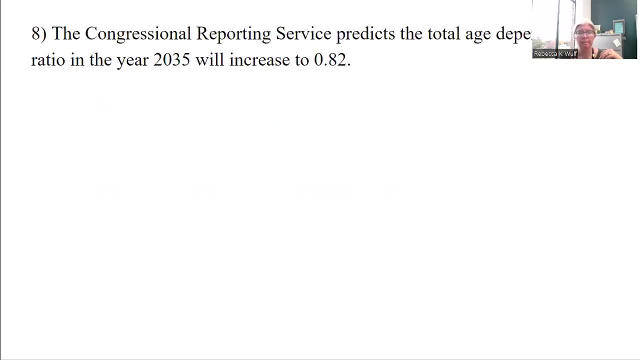 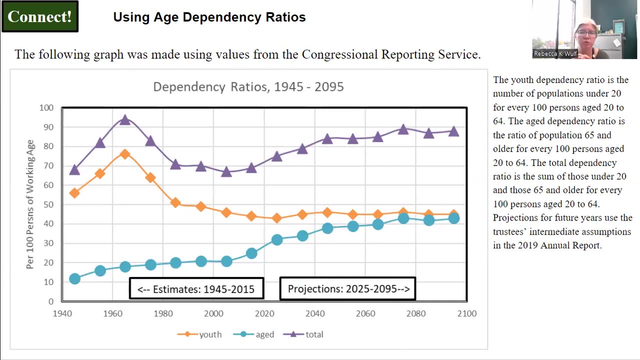 Putting the two groups together. I'm going to skip over these slides. These slides are available online And Professor Becky runs through some of these values. I do want to talk a little bit. I'd like to talk a little bit about this picture that's on one of the next pages. This will help. 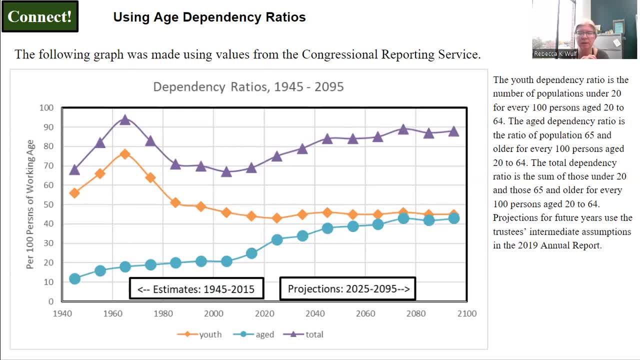 with one of the final parts of our homework questions. This gets us thinking a little bit deeper Now. we just looked at one particular group of students And we're going to look at one of the other groups of students, And we're going to look at one of the other groups of students, So I'm going to 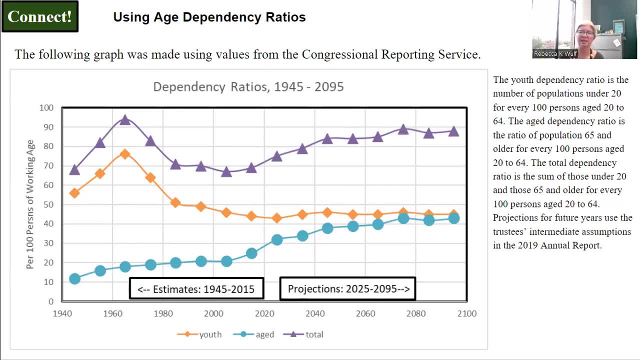 I'm going to look at one of the other groups of students And I'm going to show you here what the United States dependency ratio looks like is. Let's take a look at the graph show 11 thinks they are going to be in his whole big paragraph there for you guys to read. 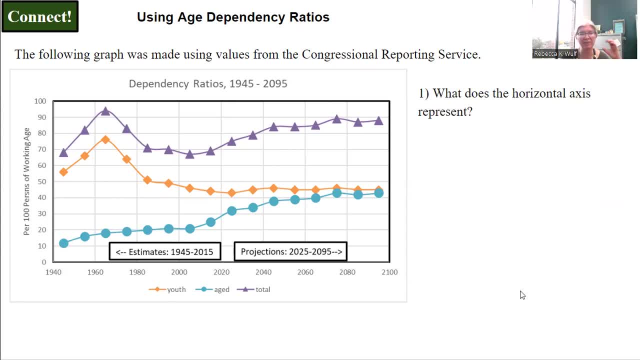 15 thinks they are going to be an. it's like to look at the graph, So I just read off some years 먹. look at the graph, So I just read off some years. that's what's on our horizontal axis: years So. let's take a closer look at the graph. So I just read off some years. that's what's on our horizontal axis. years: the project for A force to meet The multiple stories that a person understands: individual growth and development. Subtract the small smartphone from the device and 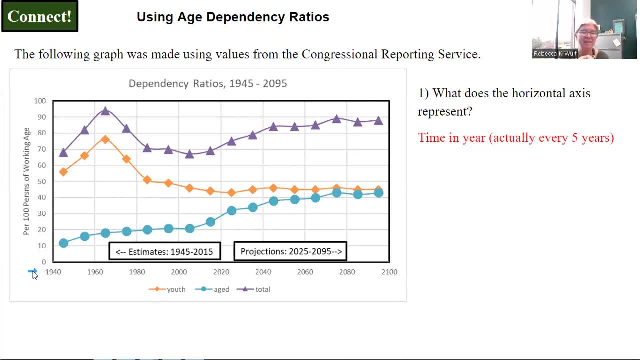 So horizontal means like the horizon, our x-axis. here we have years The vertical axis. that's our up and down axis. Oh, my axis actually has a little typo on it. I hope I fix that. in the book It says: per 100 persons of working age. 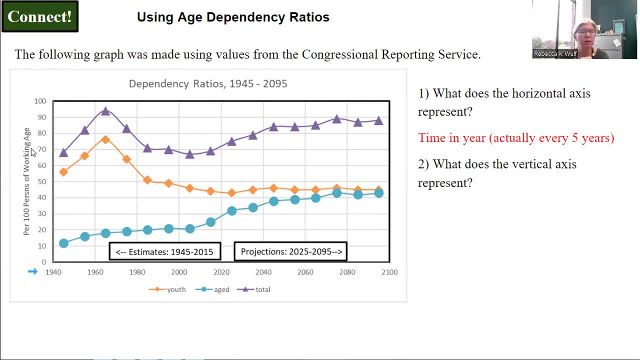 So what is this? It says 10,, 20,, 30,, 40. You might think they're percents, but, just like in the example I did a second ago, it's not a percent, It's a per 100 of working age. 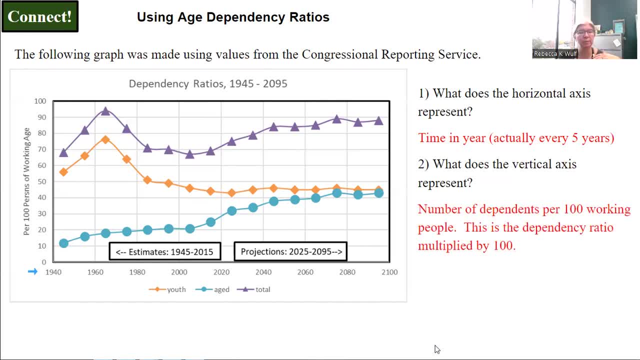 So our number of dependents for every 100 working people. That's what we're going to measure as we look at the dots and triangles and diamonds in this graphic. So let's look at one, Let's look at 2021.. Now I have three different lines. 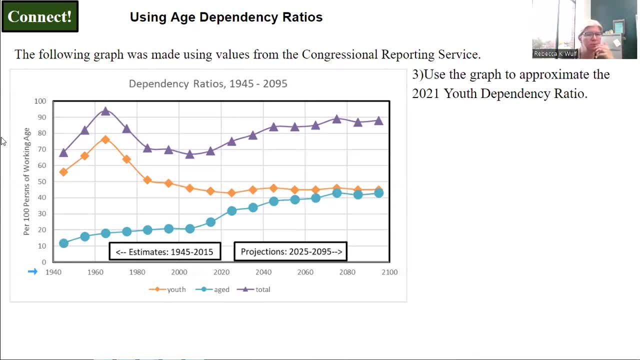 Which line do they want me to look at? Let's read the instructions here. 2021: youth tax Dependency ratio. So youth is the orange, one kind of diamonds. 2020 is marked very clearly. 2021 would be just past that. 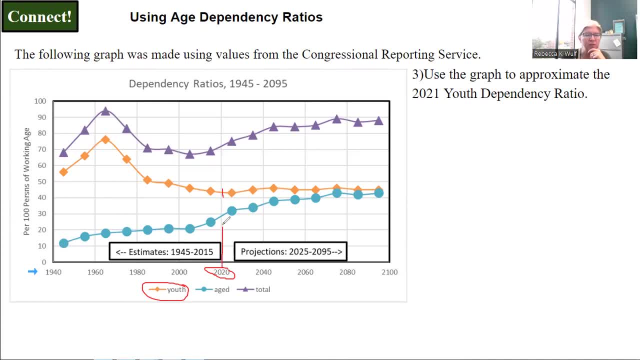 So about there. And then of course I need to look over and see what the corresponding y value for that x value is. So I'll get my line. Try to get my line nice and straight here, or not. Changed my tools in Zoom just a little bit. 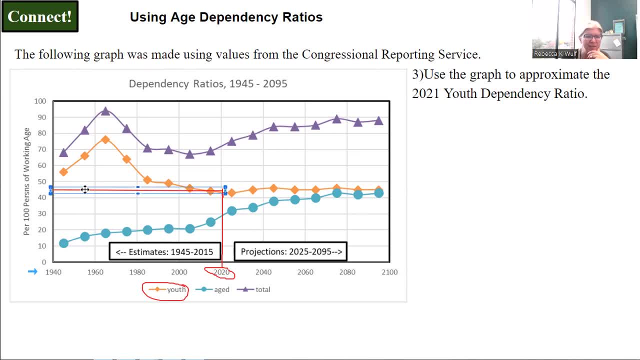 So there Probably A little bit high there. Let's see Someplace between 40 and 50. It looks like a little under 45, but definitely over 40.. You know, this is a little tiny picture in your book. 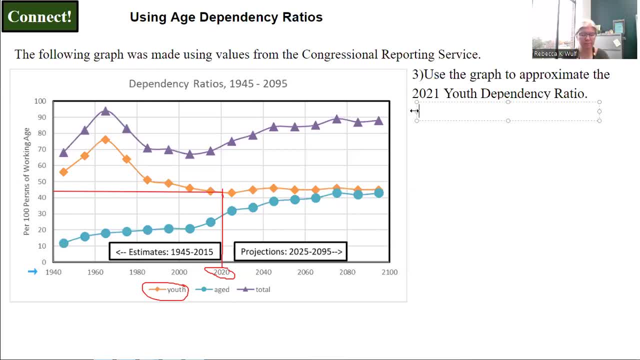 I'm going to say 43. But in this class we don't just give a number. 43 meaning what? So 43 meaning 43 dependents, Or 1%, 100 workers. Let's see what AnswerKey guys said before I go on here, because I'm going to put the answers up as I go. 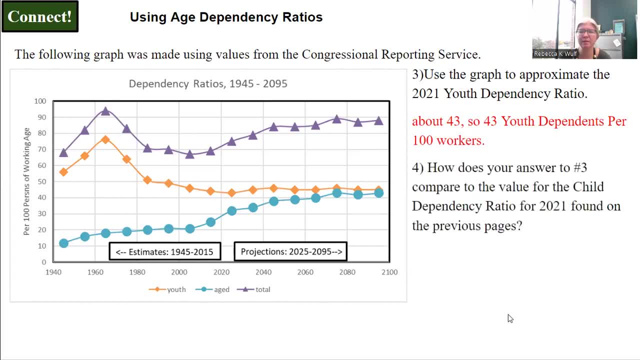 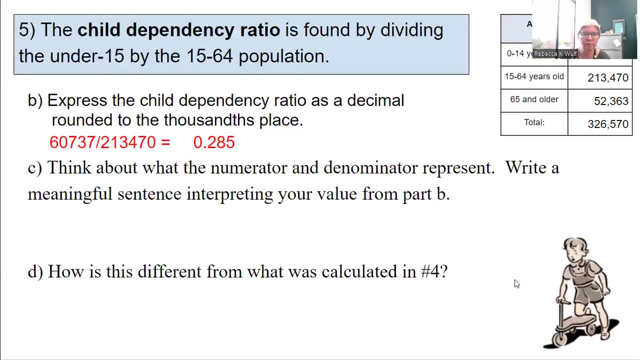 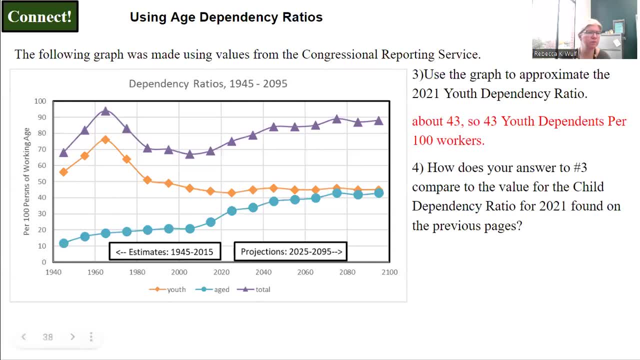 0.285.. Is that what we were just looking at? 0.285.. Is that what we were just looking at? 0.285.. So we got 0.285.. Child dependency: I'll put CD for child dependency. 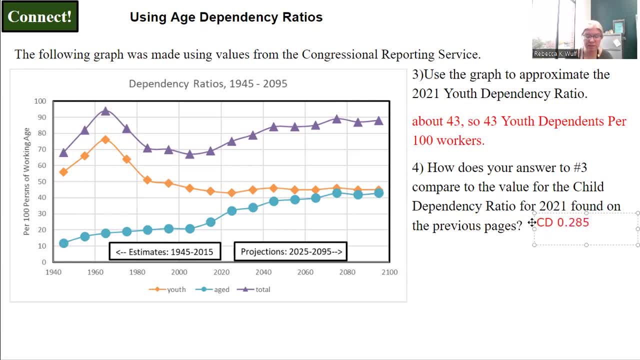 0.285, which I said was 28.5 out of 100. So we can see how does it compare. Well, this child dependency is lower than this youth dependency. Child youth, child youth- are they the same thing? 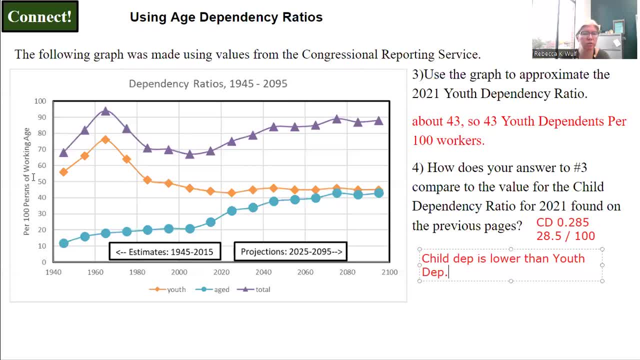 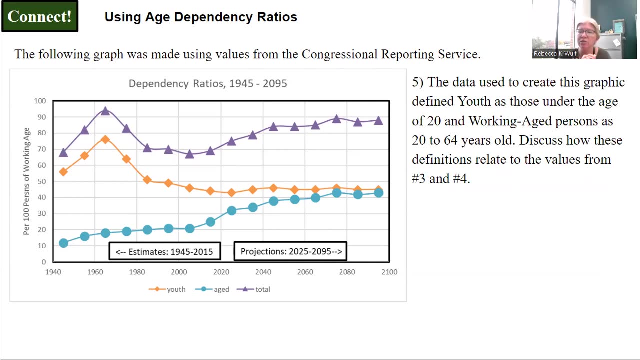 Apparently not. Let's look at the next question. AnswerKey guy said it the other direction. He said youth is higher than the child. Ah, the data used to create this graphic define youth as those under the age of 20.. So youth are under 20.. 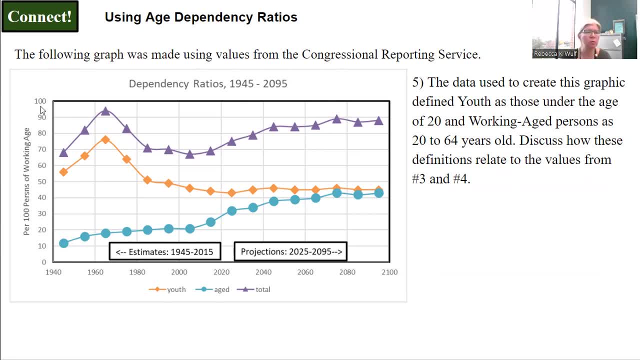 Okay, that's a different population than we work with. We said that child was under 15. And we said that workers were 15 to 64. And I usually gloss over that when I'm teaching it in class, But I hope that some of you are thinking. 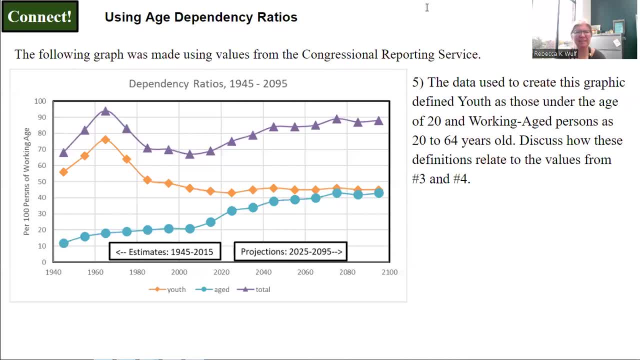 um, we're thinking 15, you're going to make these kids work at 15.. I know I worked at 15, but uh, I wouldn't think of a 15 year old as typically supporting, you know, a whole family or anything like that. 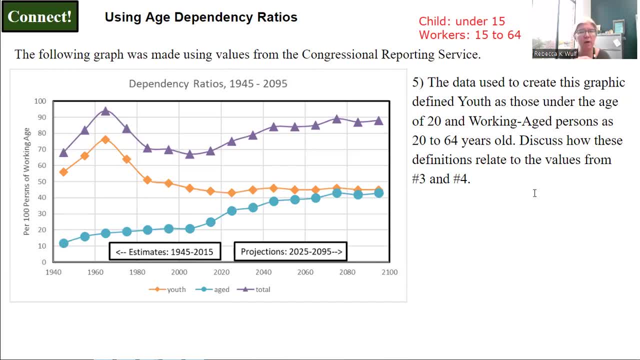 So youth defines it as 20.. Now, if the cutoff for being a kid is 20, that also means the cutoff for being a worker is 20.. Now let's think about how that would impact our ratio. So they had youth dependence over workers. 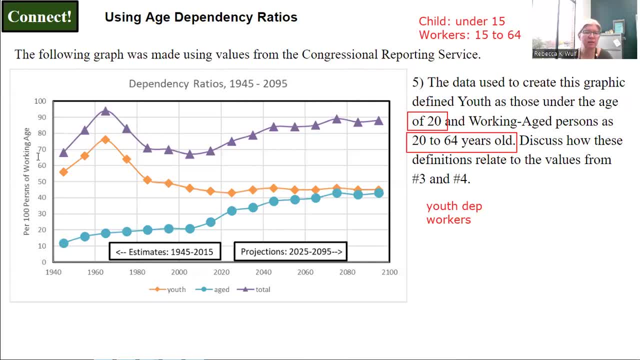 If we increase the, the children's age, right then what's going to happen? You're going to have more kids, So this value on top it's going to go up. We're going to have more Uh, child- we call them youth here, but more children dependence. 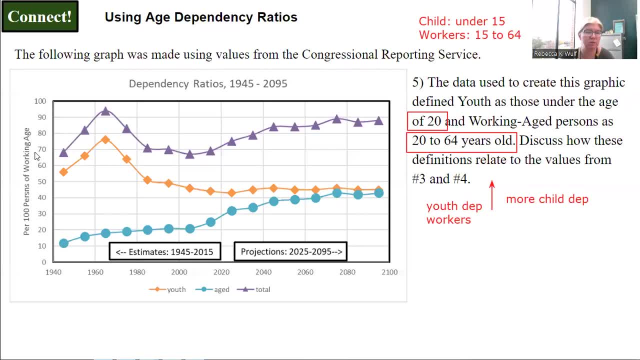 They're going to stay dependent until they're 20. by this definition. That impacts something else too, doesn't it? If they're not working, then the working group here. this number is going to go down, So we're also going to have fewer working age persons. 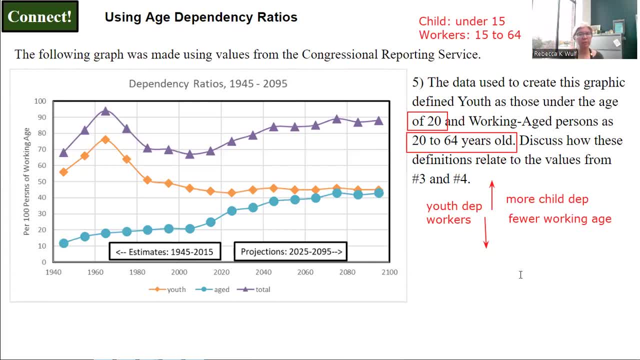 So that ratio is being pulled from both ends: The top number is getting bigger And the bottom number is getting smaller. So overall we see, uh, this value 0.43 is quite a bit larger than our 0.285, just by changing those ages by a few years. 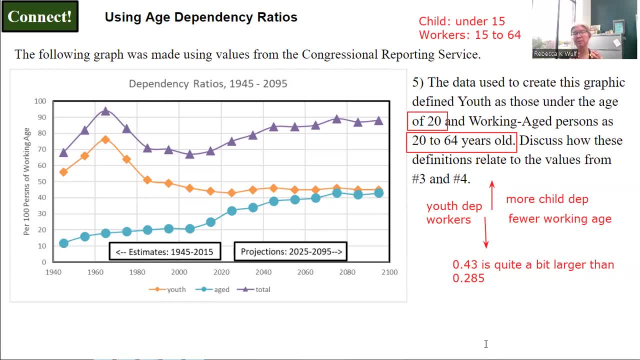 Now my students' homework. I have you think about something very similar with retirees. What if we change that retirement age? Well, keep in mind that retirement age is going to be a little bit longer. Retirement age is going to affect two things in the ratio, the two things that are in the ratio.